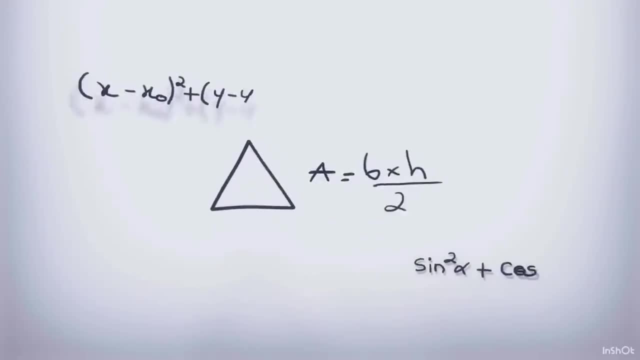 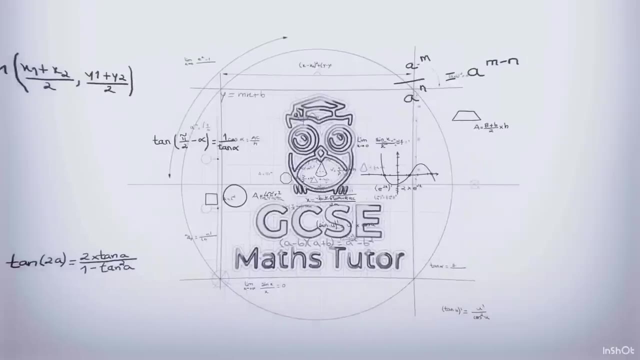 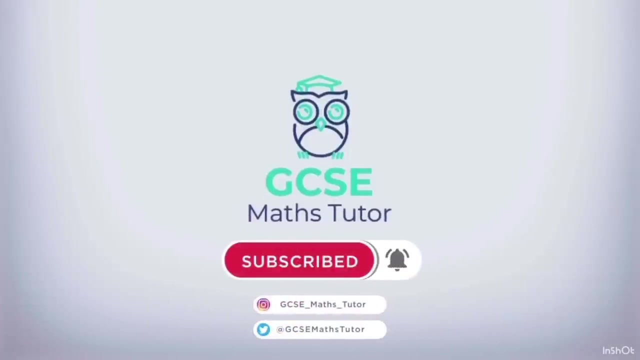 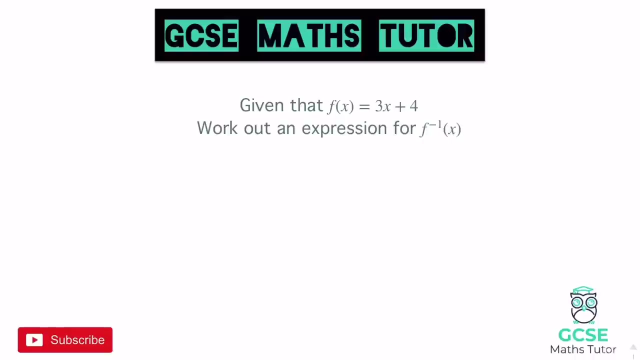 Okay, so we're going to have a look at some inverse functions. It says here: given that the function of x equals 3x plus 4, work out an expression for f minus 1x, which means the inverse function. Okay, so we're going to have a look at doing this. So grab a piece of paper. 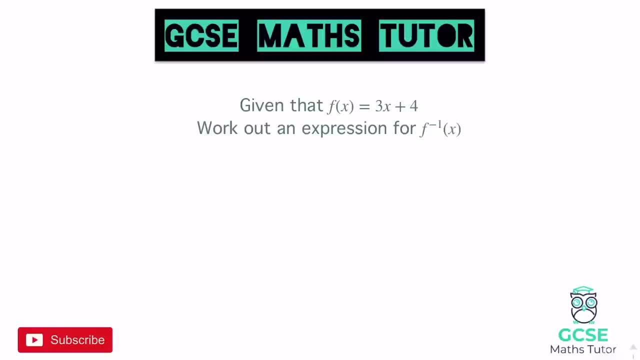 grab a pen, make some notes and we'll start with this question. So the inverse function of x just means essentially what is the opposite or the reverse of this function. Now, the function at the moment, 3x plus 4,, just means that whatever number you put in, it gets multiplied by 3,. 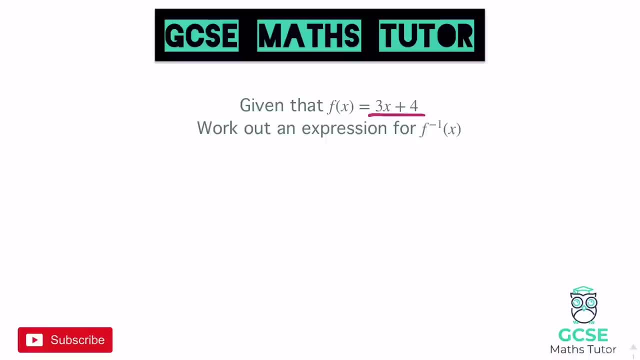 and then you add 4.. And if we think logically, the reverse of that would be taking away 4 and dividing by 3.. But we're just going to have a look at a process for actually working out a method for how we can actually go about writing this expression out for this inverse function. 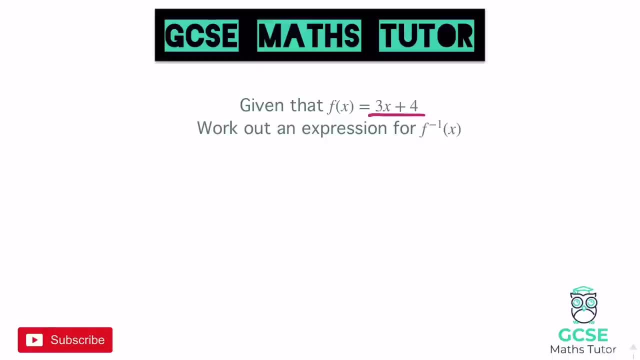 Now, it's just personal preference. There are lots of ways of doing this. This is just the way that I like to do it. Now, instead of writing the function of x equals 3x plus 4, I like to just write y equals 3x plus 4.. So I write: y equals 3x plus 4.. And now what I do is I rearrange it to. 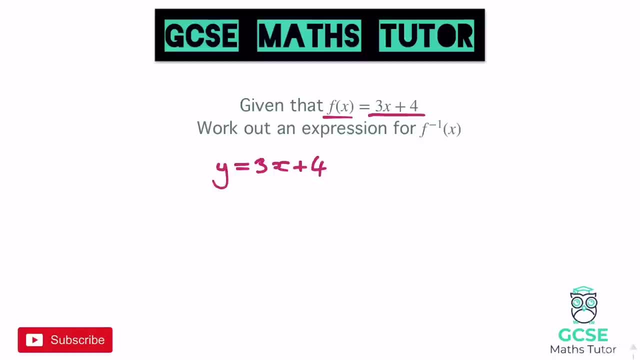 make x the subject. So if I want to make x the subject, first thing that I do is I'm going to have to take away 4- here. Obviously, it's just rearranging equations So you can always have from both sides- would leave you y minus 4 equals 3x, And then to get x as the subject. 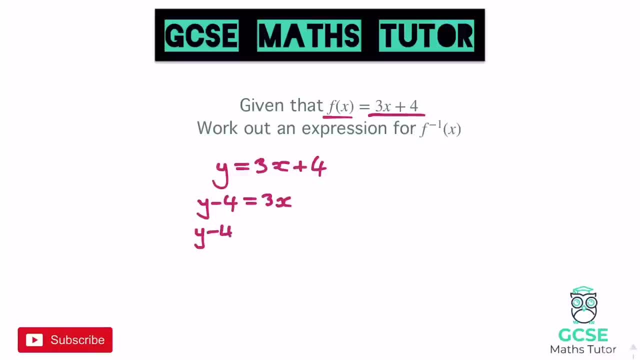 we would divide by 3. And we'd get y minus 4. all over 3 equals x. Now, obviously the y I only put in place there just to help me rearrange it. Obviously this isn't a very nice piece to. 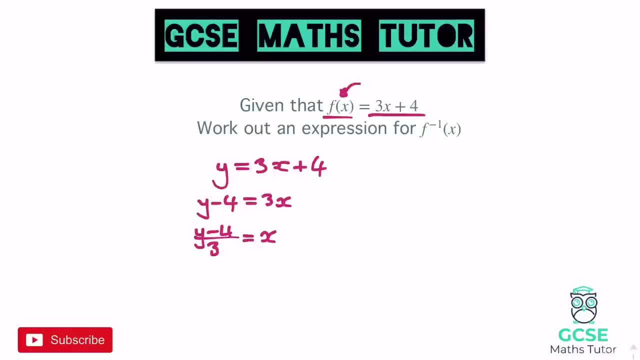 rearrange f of x. So it's just easier just to replace it with a letter. And what we're going to do here now is just swap the x and y over to put the x back in, And that would leave us with x minus 4 over 3 rather than y minus 4 over 3.. And that equals the inverse function of x. 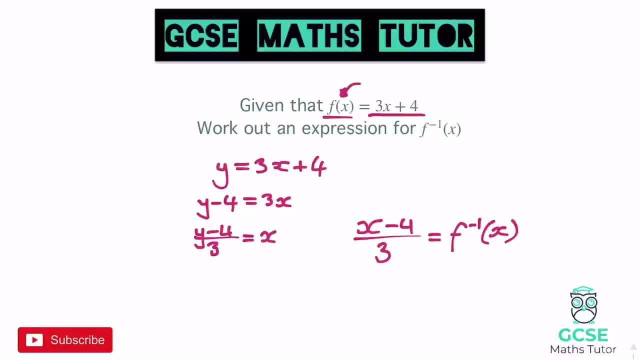 OK, And think back to the logical idea there. We said x would help you to reverse times in by 3 and adding 4.. You would take away 4 and divide by 3.. And that's what's shown there in the inverse. 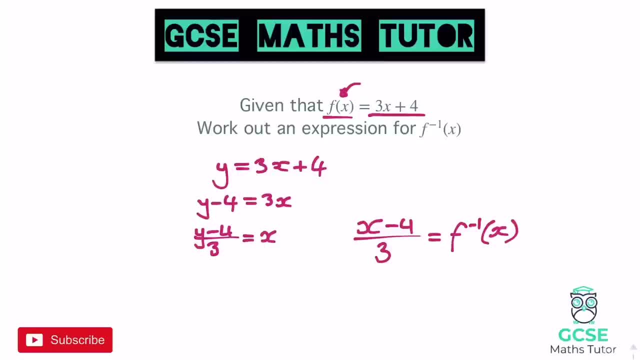 function x, take away 4 and then divide by 3. And that is our inverse function. OK, So what we're going to do is write y equals instead of f of x, make x a subject and then swap x and y, So three. 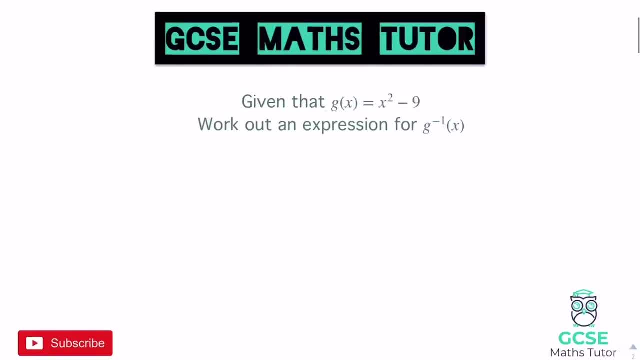 steps there with some rearranging. Let's have a look at another one. OK, So in this question I've got g of x. OK, So it's exactly the same as f of x. It's just a different function with a. 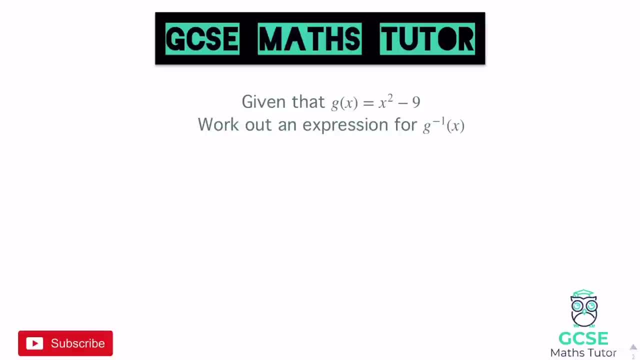 different letter. So sometimes you might have this OK, But don't let that throw you. It's just a different letter for the function. So, given that g of x equals x squared minus 9, work out an expression for the inverse function of g. So same again. I'm going to replace g of x with y, So y. 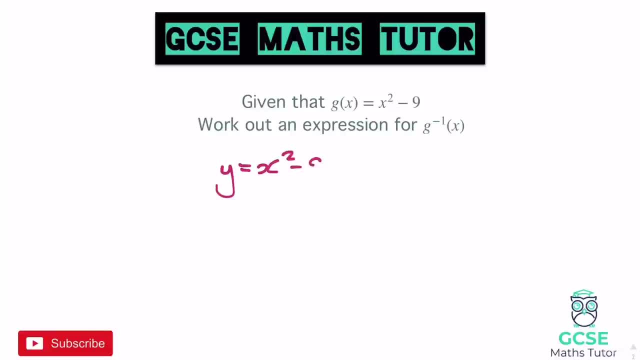 equals x squared minus 9.. And let's just make x the subject. Add 9 to both sides. We get y plus 9 equals x squared. And then to get x as a subject, we're going to have to remove the square. So we're going to have to square root both sides And we get the. 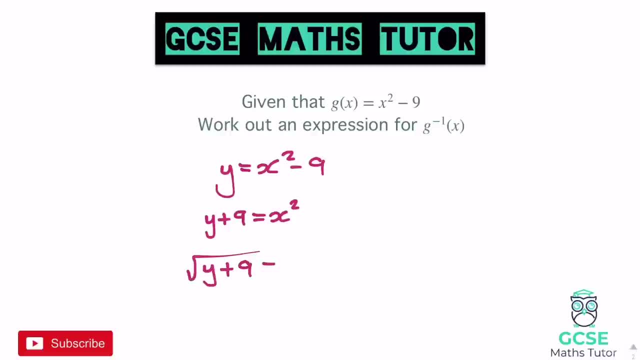 square root of y plus 9, equaling x, And then, to finish it off, obviously just swap the x and y again, So you get the square root of x plus 9 rather than y plus 9.. And that is equal to the. 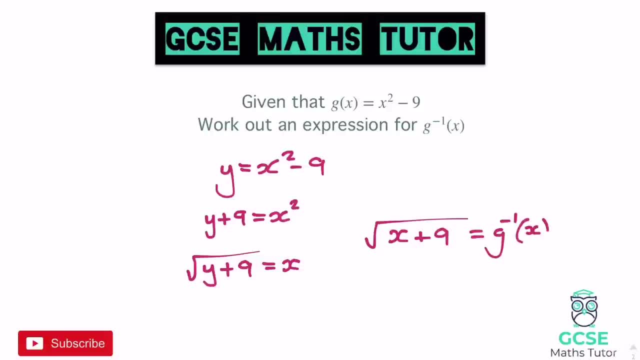 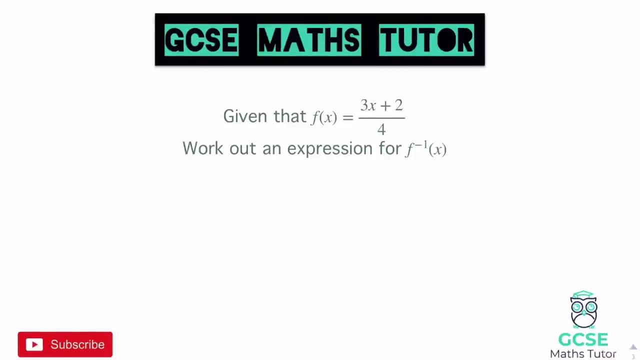 inverse function of g. OK, So just write that out: Equals the inverse function of g. There we go: The square root of x plus 9.. One more question before you have a go. OK, So we've got some fractions involved in this. 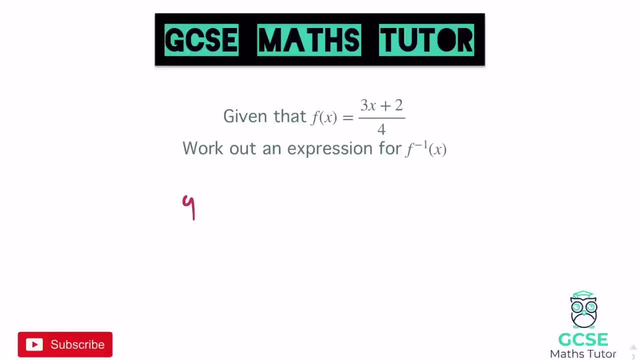 question as well, But we're going to treat it in exactly the same way. So I'm just going to write: y equals 3x plus 2 over 4.. I'm going to rearrange it to make x the subject. So first things first. 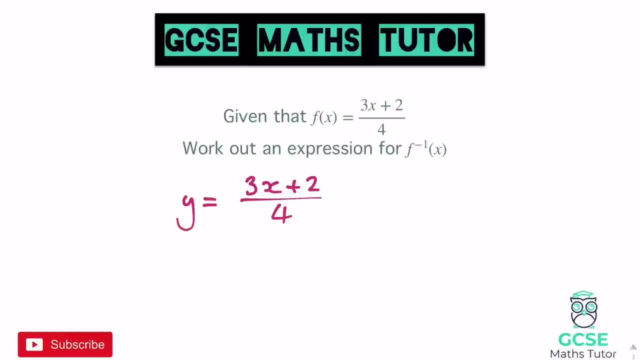 we're going to have to get rid of this divide by 4 on the bottom. So let's times that over. So timesing both sides by 4 would give us 4y equals 3x plus 2.. Subtract 2 from both sides. 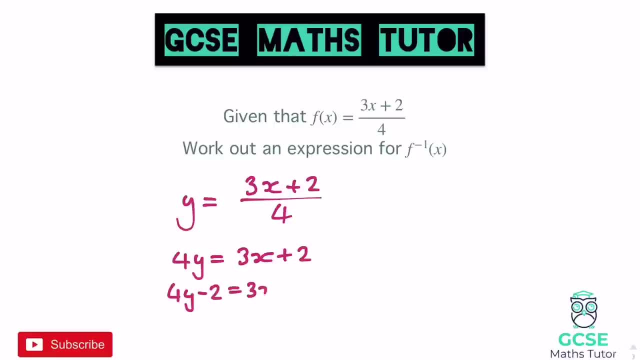 So 4y minus 2 equals 3x, And then divide both sides by 3. So it'd be 4y minus 2, all over 3 equals x. And then again, finishing that off, just swap the x and y over, So, rather than it: 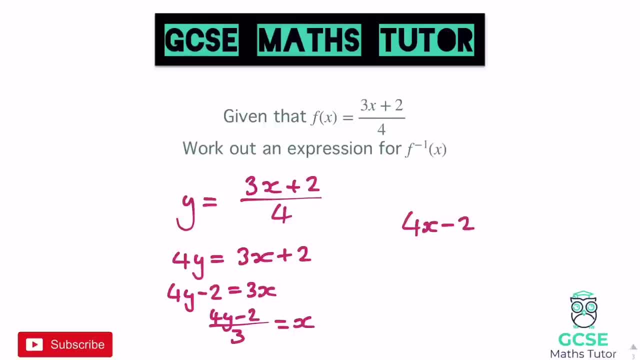 being 4y, it'd be 4x minus 2 all over 3.. And that equals the inverse function of f. OK, So swap the f of x or g of x for y equals, Rearrange it to make x the subject, And then just swap your x's and y's back over And you'll get. 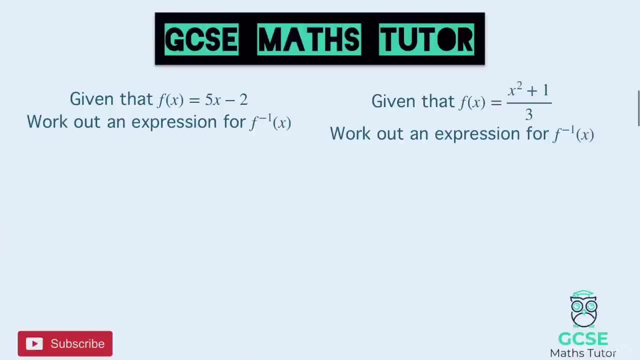 your inverse function. Here's some for you to have a go at. So have a go at these two. Pause the video there. We'll go over the answers in a sec. OK, So for the first one swap that for y equals. 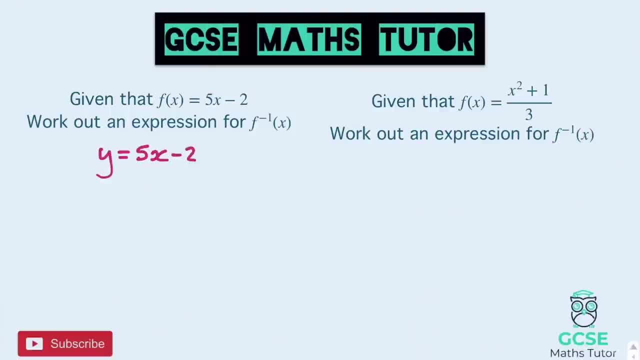 So y equals 5x minus 2.. OK, Rearrange it So we get y plus 2 equals 5x Divide by 5.. y plus 2 over x, And then swap your x and y, So x plus 2 over 5 equals the inverse function of f, which I'm going. 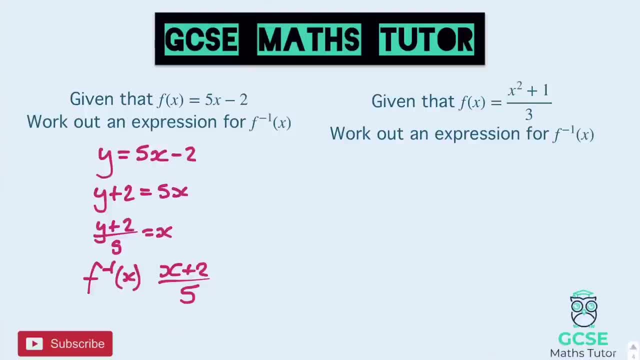 to put at the start this time. So f minus 1 of x, the inverse function equals x plus 2 divided by 5.. And there's our final answer. OK, On to the next one. So write it as y equals, So y equals. 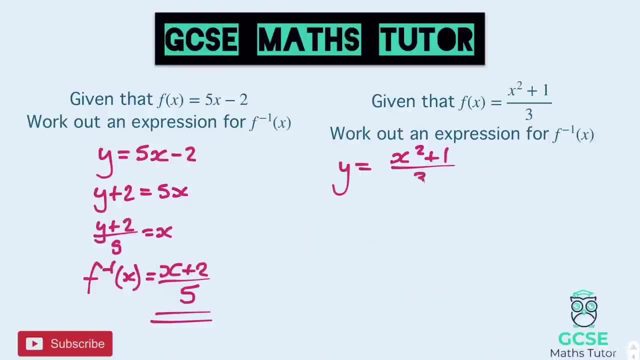 x squared plus 1 over 3.. Just as a side note, you could actually just swap the x and y here and make y the subject again, But I'm just going to stick with the same method that I always use here. So times both sides by 3. We get 3y equals x squared plus 1.. Take away the 1 from both sides. 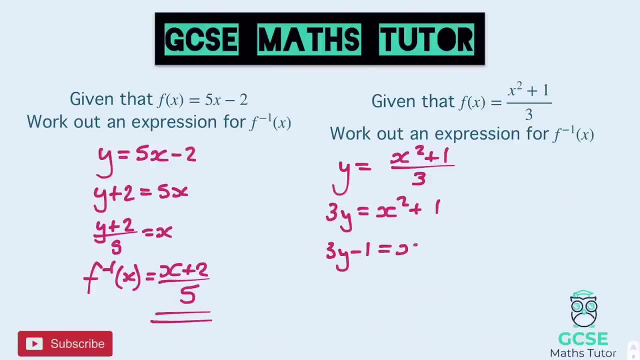 So 3y minus 1 equals x squared, And then square rooting both sides would leave us with the square root of 3y minus 1 equaling x, And then finish that off. Swap your x and y, So we have 3x minus. 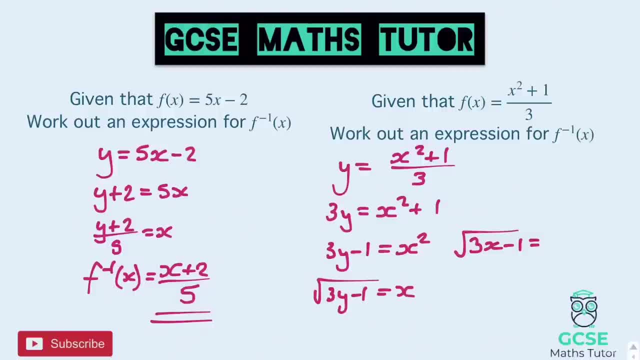 1 to the square root, And that equals the inverse function. Over, Right, There we go, And there's inverse functions, And there's our second one, Right, Let's have a look at something else. OK, So this question says: given that f of x equals 2 brackets, 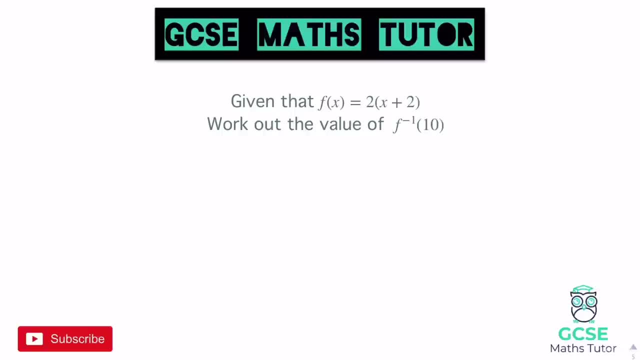 x plus 2, work out the value of f minus 1 with a 10 in there, So that f minus 1 still means the inverse function, But with a 10 in there means it's going to want us to do something with that. 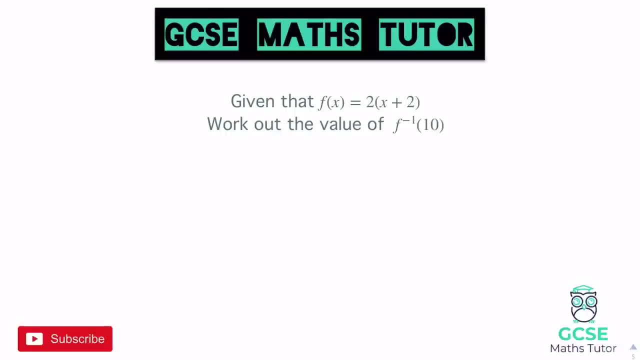 in a second. We'll talk about that once we get the inverse function. But first things first. we can see this inverse f, So let's find an expression for the inverse of f. Now, straight brackets this. We need to expand these brackets. So let's expand that straight away when we write. 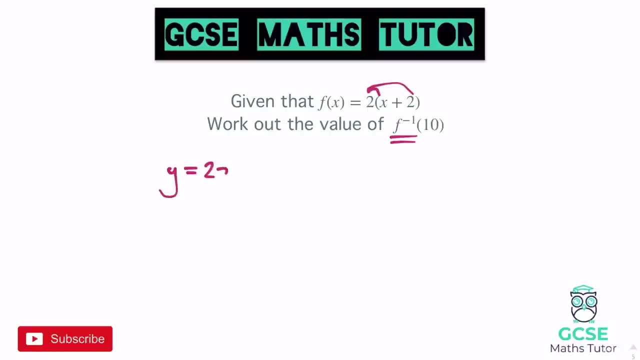 y equals. So y equals 2 times x, which is 2x, And 2 times 2,, which is 4.. So plus 4.. And let's find the inverse function. So subtract 4 from both sides: y minus 4 equals 2x, Divide by 2. We get. 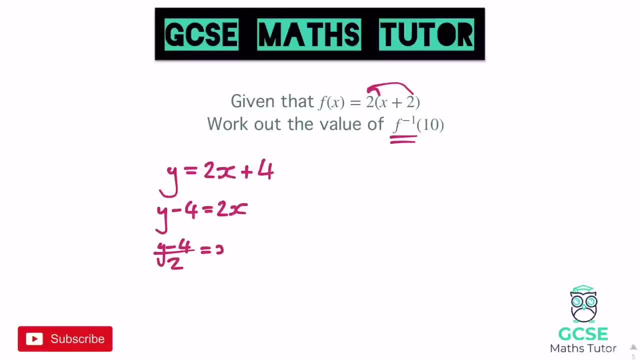 y minus 4 over 2 equals x. And let's write our inverse function, So f minus 1 of x equals x minus 4 over 2.. Now, whenever you're given a number in the brackets here, it just means it. 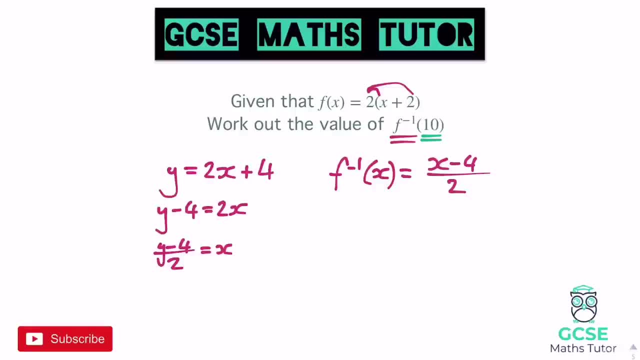 wants you to replace x with the number. That's why it says: work out the value. So what I'm going to do is I'm going to sub in x equals 10 into my little expression here. So I've got x minus 4 over. 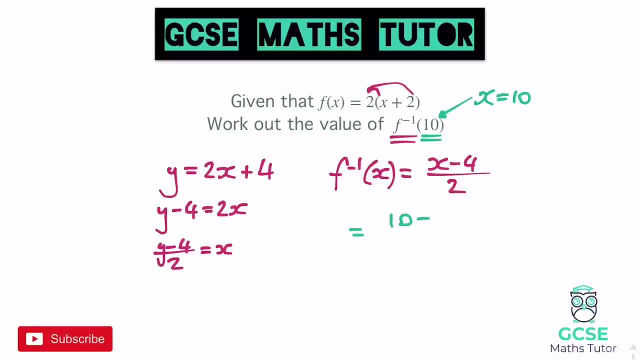 2. And that's going to become 10 minus 4 over 2.. 10 minus 4 equals 6.. So it's 6 over 2, which gives me a value of 3.. OK, So find the inverse function. 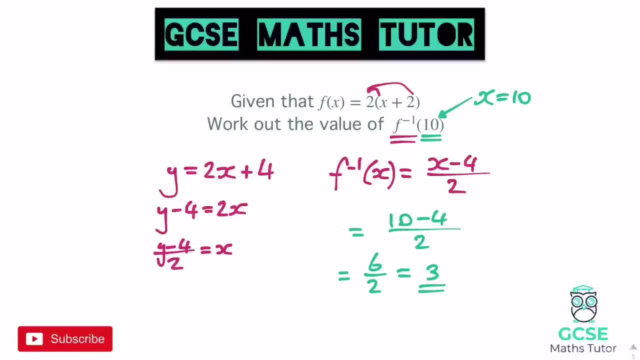 And then sub that number in. There is another process to actually go about solving this, But I think it's a good process just to write out the inverse function and then sub it in, Because there's two elements of the maths going on there, rather than applying a little trick here. OK, So, 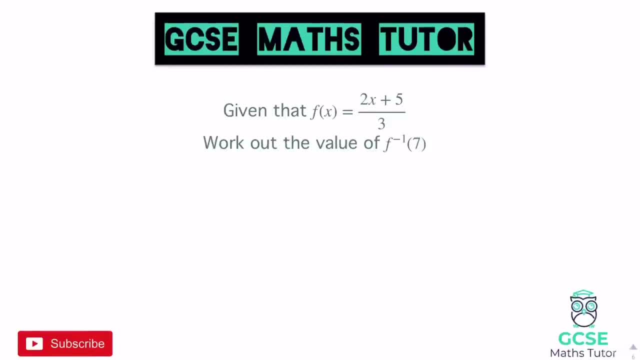 let's have a look at one more before we have a go. OK, So given that f of x is 2x plus 5 over 3, work out the inverse function of f when we put 7 in. So don't forget once we get the inverse. 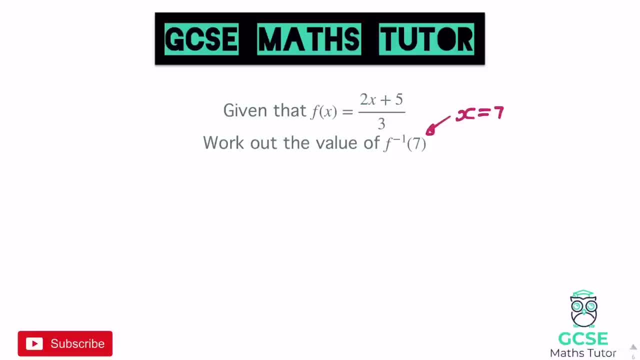 function we're going to sub in: x equals 7.. OK, But let's actually find the inverse function first. So y equals 2x plus 5. Over 3. And let's rearrange that: So 3y times both sides by 3 equals 2x plus 5.. Subtract 5 from 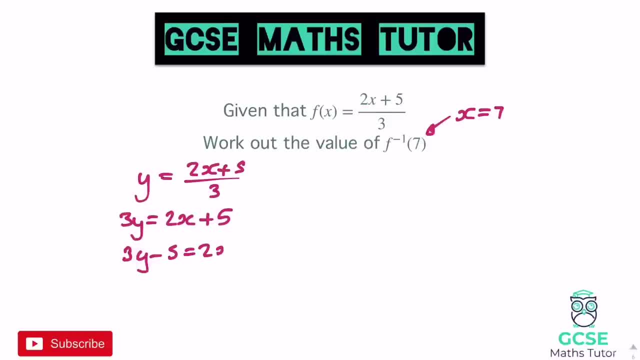 both sides. 3y minus 5 equals 2x, And then divide by 2.. 3y minus 5 all over 2 equals x, And let's rewrite that out. So the inverse function of f equals 3x minus 5 over 2.. 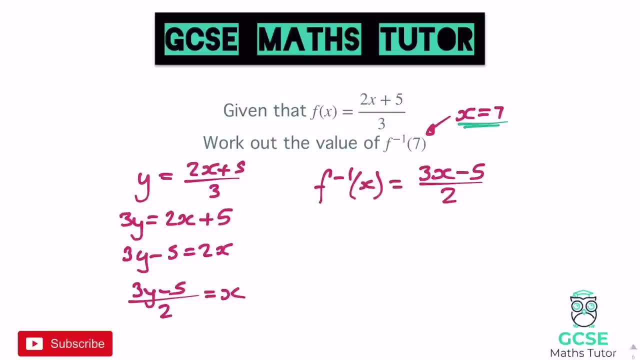 OK, So subbing in x equals 7.. Let's put that in. What do we get? We get 3 times 7.. I'm going to write it all in 3: lots of 7 minus 5 over 2.. 3 times 7 is 21.. So we have 21 minus 5 over 2.. 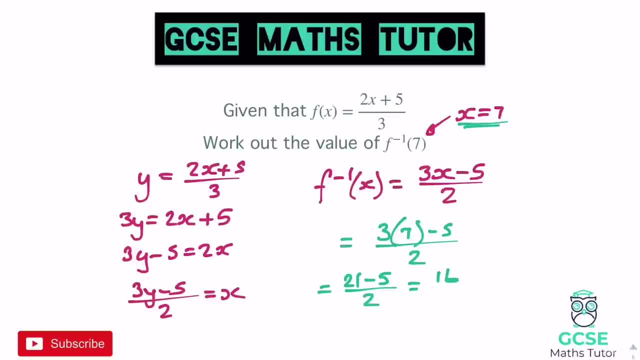 21, take away 5 is 16.. So we have 16 over 2.. And 16 divided by 2 equals 8.. So you might be able to do some of those steps in your head there, but just showing you all the process of subbing that in. 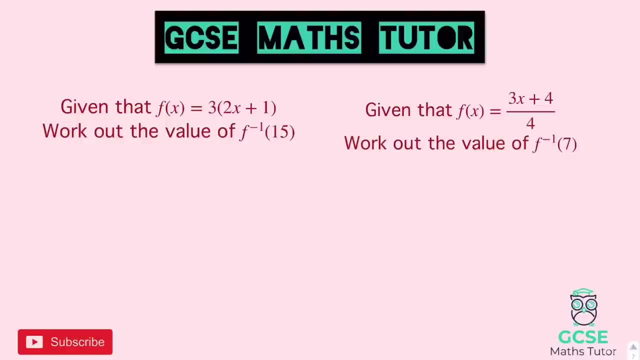 to that final answer. OK, So here's something for you to have a go at. OK, So there's two questions. Have a go at both of these. Pause the video there. We'll go over the answers in a sec. OK, So for the first one, y equals, and let's expand this bracket. So 3 times 2x is 6x. 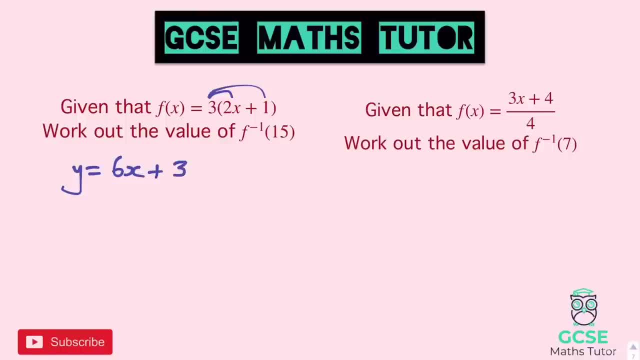 3 times 1 equals 3.. So plus 3.. Rearranging that, we get y minus 3.. I'm going to do it in two steps. One step over: 6 equals x And let's write that function out: So f minus 1 of x. 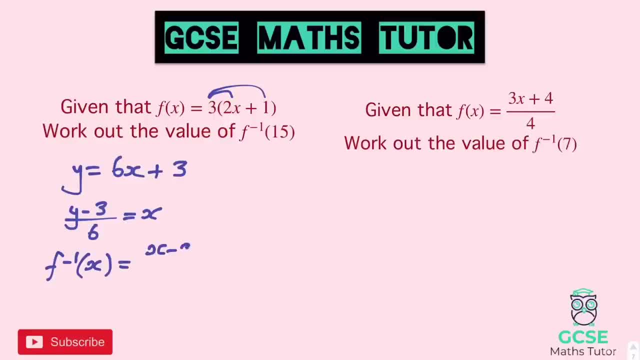 equals x minus 3 over 6.. And now let's sub that number in, So x equals 15.. So what do we get? We get 15 minus 3 over 6.. 15 take away 3 is 12.. So it's 12 over 6,, which equals 2.. And there's. 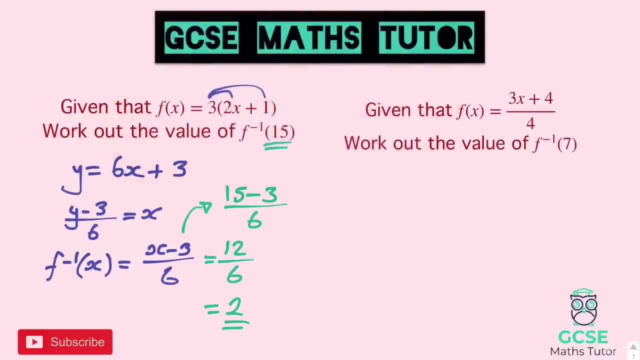 our final answer: 2.. And on to the next one. Let's write this out: So y equals 3x plus 4 over 4.. And let's rearrange this So we get 4y when we times by 4.. Then we're going to take away: 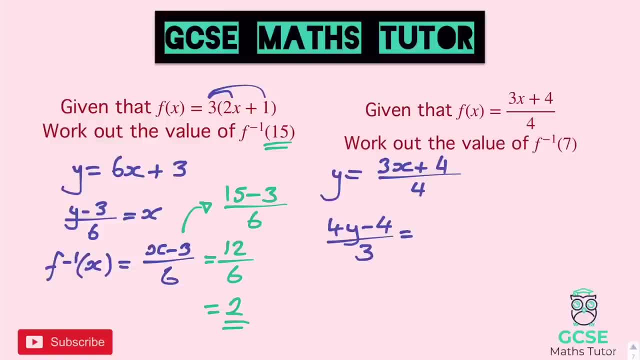 4. And then we divide by 3. And that equals x. OK, So I've obviously done that in a very short step there. But f minus 1 of x equals 4x minus 4 over 3.. And then the number it wants us to sub. 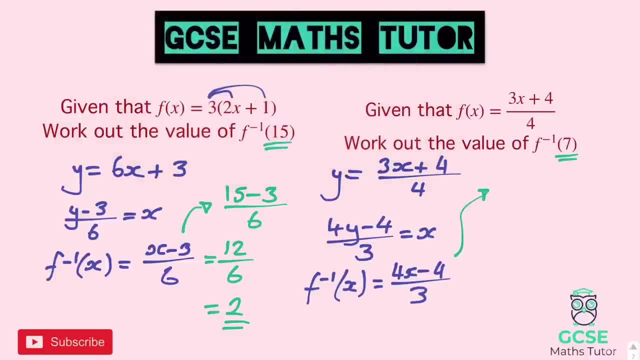 in. there is 7.. So if we sub 7 in, let's see what we get. We get 4 lots of 7, which is 28.. So we get 28.. And then we get 4 lots of 7, which is 28.. So we get 4 lots of 7,, which is 28.. So we get.